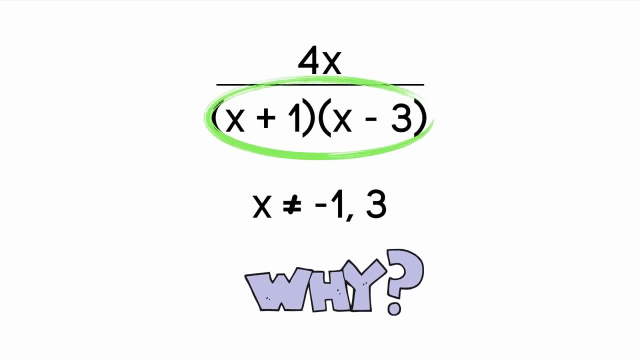 So when we work with rational expressions, we have to state restrictions on the denominator. But why is that? Let's take a look at the example. Say, I have a rational expression- 2 over x plus 1. And I need to see where the expression will be undefined. Undefined means: 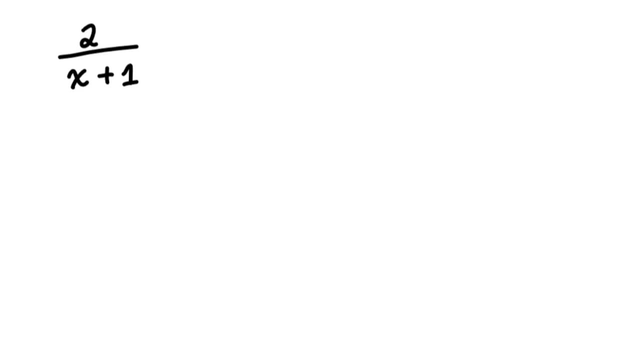 it will have no meaning, It will have no possible value. Say: I want to evaluate this expression for x equals 2.. Let's try it So: if I sub in 2 for x, so x plus 1, and then 2.. Consequently, now my x is 2 plus 1.. 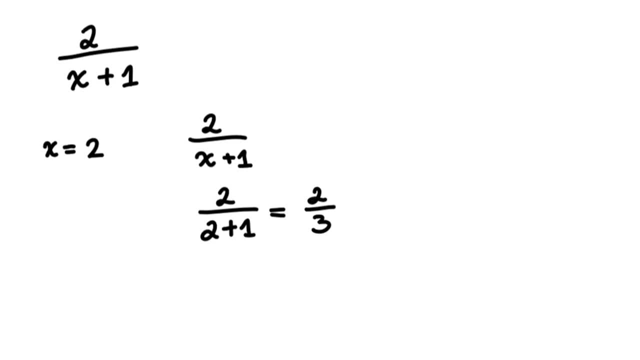 I will get 2 over 3.. So when x is equal to 2, the output value, the evaluated value of the expression, will be 2 over 3.. What if I want to evaluate my expression for x? x equals negative 1? So then, if I take that same expression and I substitute negative 1, 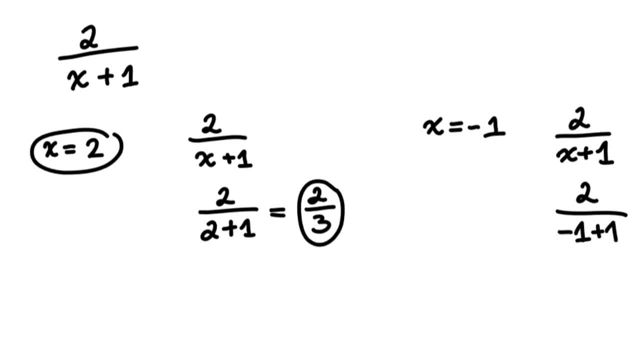 into the denominator. what happens here? We get a 0. So we end up doing 2 divided by 0. Is that possible? It's not. We cannot divide by 0. So therefore, we cannot allow the denominator to equal to 0. 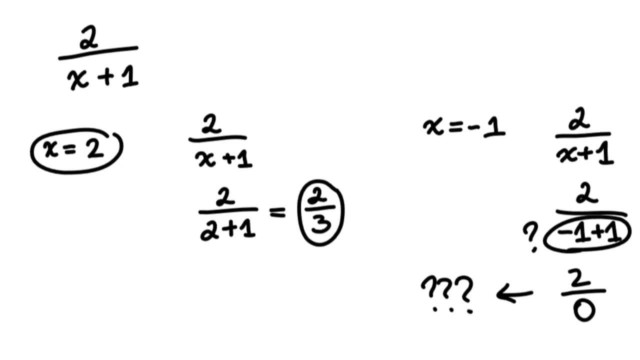 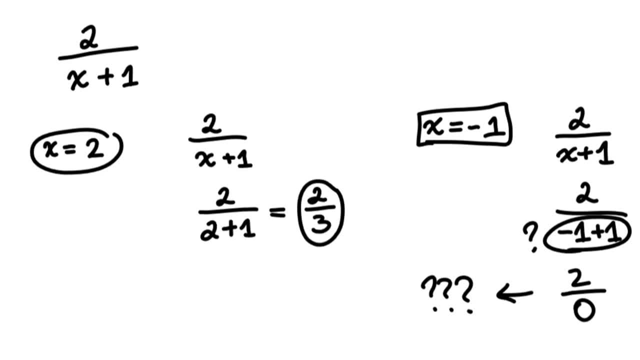 it will make my denominator 0. So if I take x minus 1, it will make my denominator 0.. So if I take x minus 1, it will make my denominator 0.. So if I take x minus 1, it will make my denominator 0.. So the 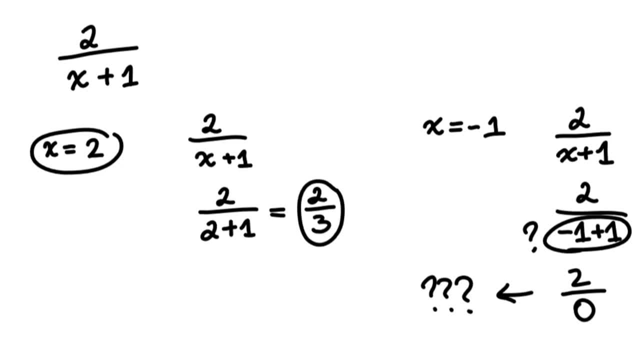 And in order for us to avoid that, we need to state restrictions on the variable in the denominator. that will make the expression in the denominator 0. So if I take x minus 1, it will make my denominator 0. So I will have a value of 2 over x plus 1.. So I will have a value of times 0.. I will be gutenberg's state, So, in addition to taking my Stepунjo-Magn stand стали mouth while editing Subtitles, Pairing My Joannaahs compensisions during the intermission, i live training. So, if this result will allow my Mara Clauizing, Be now our Debate. your questions, Any questions, or Killing, please feel welcome. 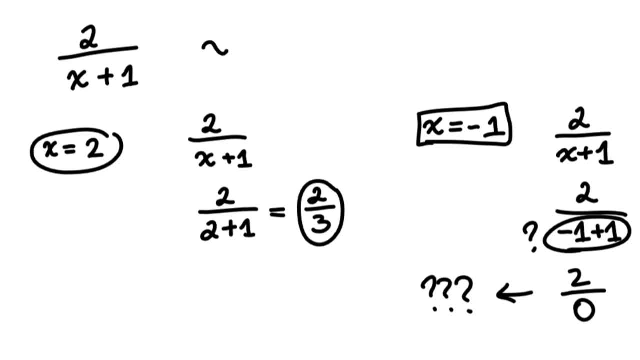 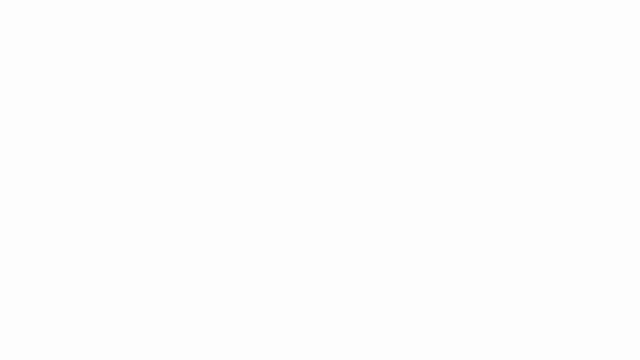 my denominator 0. So the restriction here will be: x cannot equal negative 1, because that's the value that will make the function, the expression, undefined. Say you want to add two rational expressions: x plus 1 over x minus 3 plus 3 over x plus 1.. You need to look at each one of those. 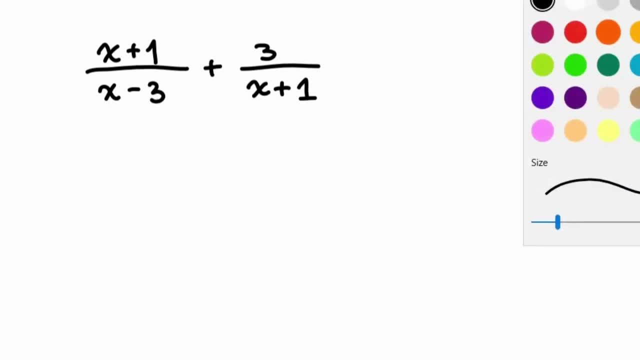 expressions and decide which value will make the denominator 0. Which value of the variable will make the denominator 0. So if I look at x minus 3, what value of x will turn that expression into a 0?? Positive 3, right. 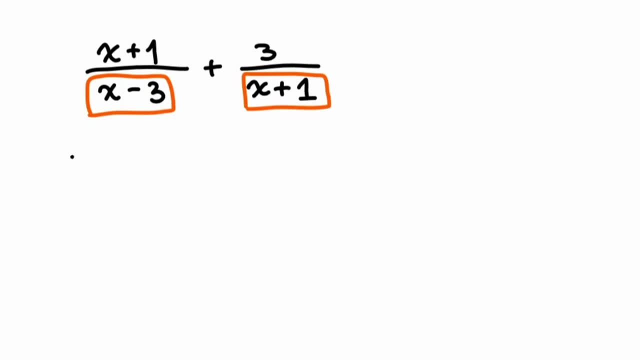 So in order for you to figure that out, you can also take that expression in the denominator and make it equal to 0 and solve a simple equation for x. So then x is 3, but we want it to be 0. So if I look at x minus 3,, what value of x will turn that expression into a 0? Positive. 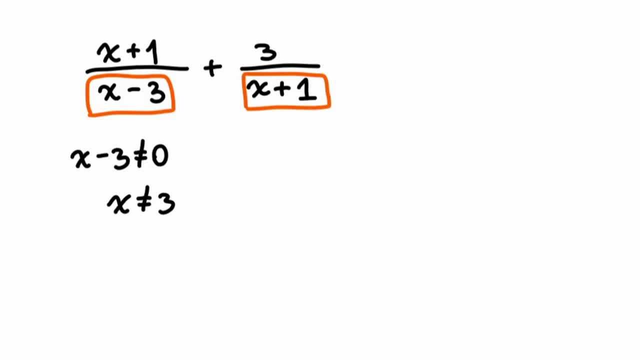 3, right? So in order for you to figure that out, you can also take that expression in the denominator and make it equal to 0 and solve a simple equation for x. So then x is 3, but we want to cross the equal sign, So we cross the equal sign. It cannot equal 3.. And for the other one: 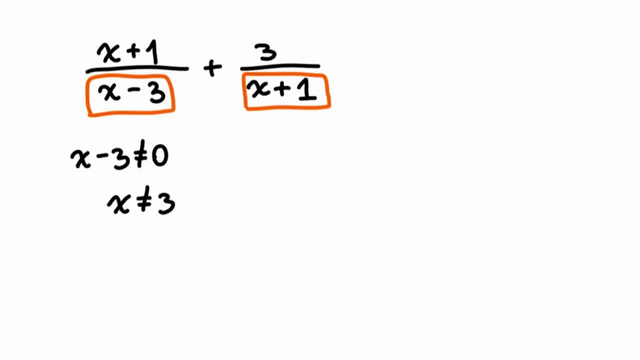 it's the same process. So x plus 1, what value of x will make this denominator? 0? Negative, 1, right, The exact opposite of 1.. In order for us to find it, we can always make it x plus 1 cannot. 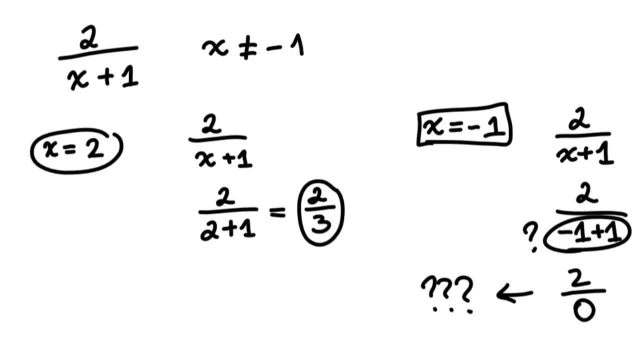 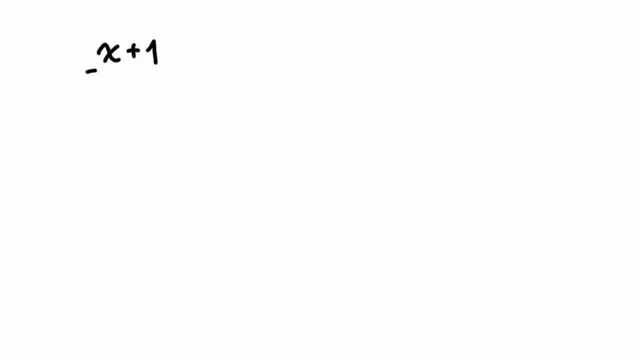 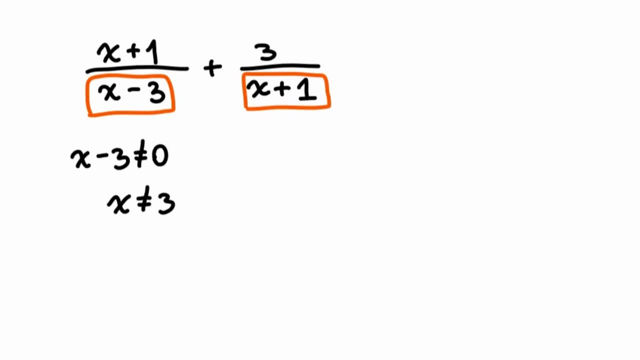 one. what value of x will make this denominator zero? Negative one, right, The exact opposite of one. In order for us to find it, we can always make it: x plus one cannot equal zero. therefore, x cannot equal negative one. See Now, when you're adding, you need to find the common denominator. 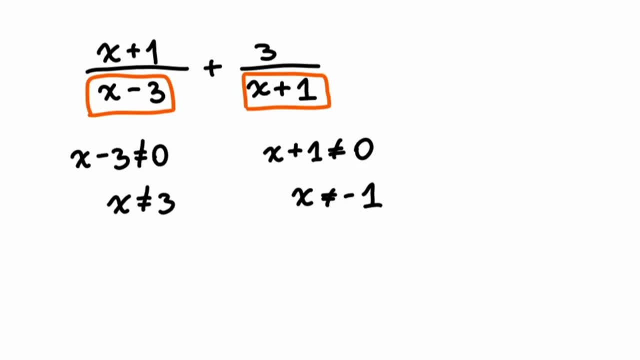 The product of the two or more factors that already exist in the denominators. But you need to state the restrictions on each one of those factors separately. Why do we not state restrictions on the numerator? Let's say you have an expression x minus one. 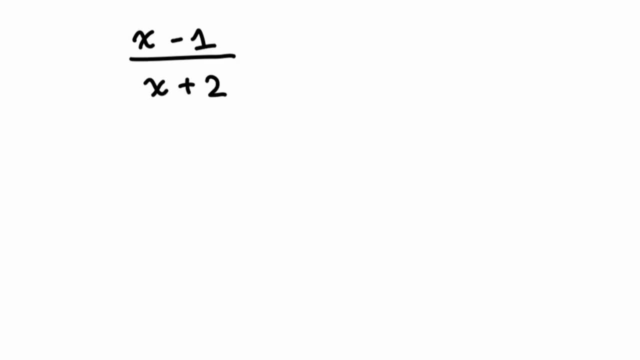 over x plus two, And you want to evaluate it for x equals positive one. Let's try to evaluate it. One subtract one over one plus two equals zero divided by three. And when you get zero in the numerator, the expression is not undefined. In fact, when you divide zero by any number, it just becomes. 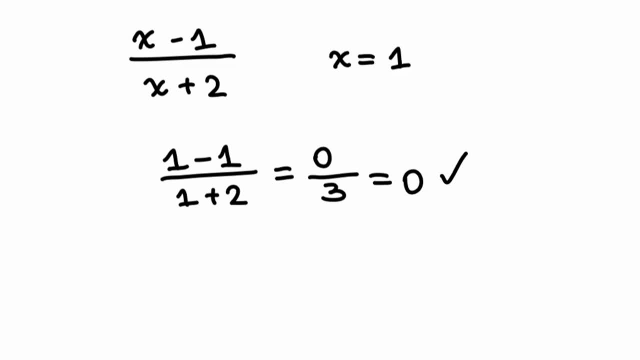 zero. So when x is one, the output, the evaluated expression, is equal to zero. So therefore, there is no need to set restrictions on the numerator, But you do need to set restrictions on the denominator. still, Let's look at this denominator and decide what the restrictions. 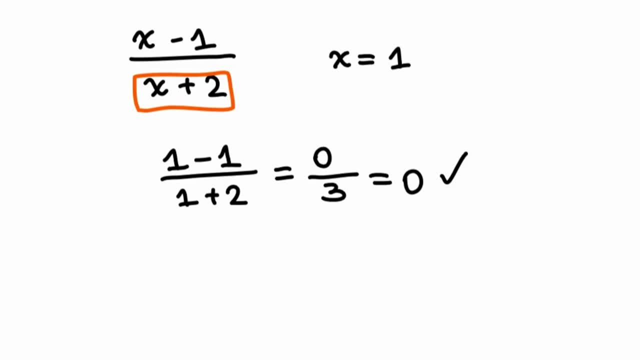 will be x plus two. what value of x will make this denominator equal to zero, Negative two. So in order for us to get it, we can set: x plus two cannot equal to zero And then x cannot equal negative two. So we'll stated as our restrictions: 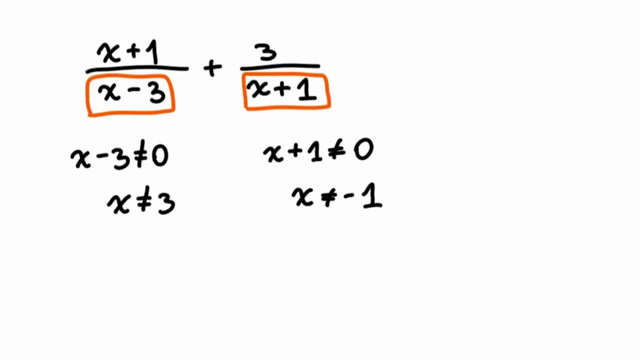 equal 0. Therefore, x cannot equal negative 1.. And then you can also take that expression in the one see. now, when you're adding, you need to find the common denominator, the product of the two or more factors that already exist in the denominators, but you need to state the. 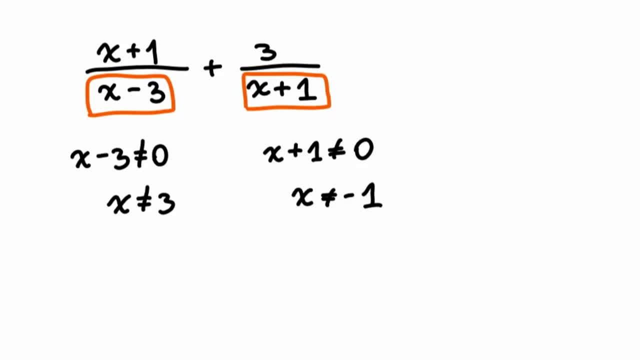 restrictions on each one of those factors separately? why do we not state restrictions on the numerator? let's say you have an expression x minus 1 over x plus 2 and you want to evaluate it for x equals positive 1.. let's try to evaluate it: 1 subtract 1 over 1 plus 2 equals 0 divided by 3. 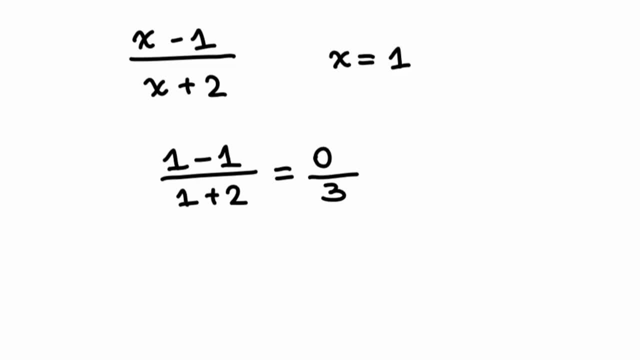 and when you get 0 in the numerator, the expression is not undefined. in fact, when you divide 0 by any number, it just becomes 0. so when x is 1, the output, the evaluated expression, is equal to 0. so therefore there is no need to set restrictions on the numerator, but you do need to set 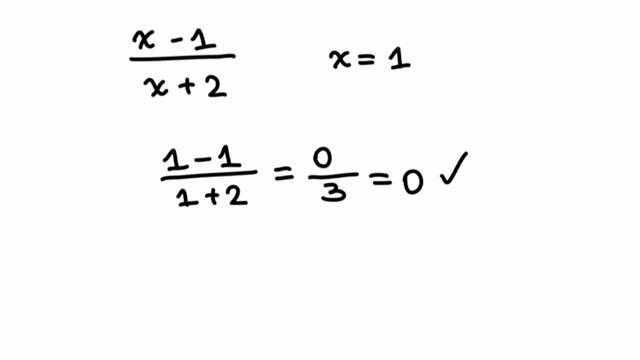 restrictions on the denominator. still, let's look at this denominator and decide what the restrictions will be. x plus 2, what value of x, will make this denominator equal to 0, negative 2. so in order for us to get it, we can set: x plus 2 cannot equal to 0, and then x cannot equal negative. 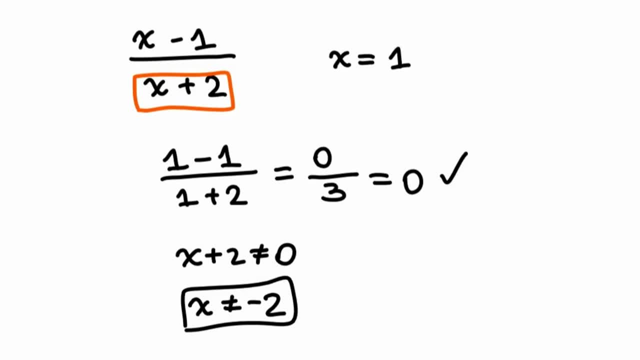 2.. so we'll state it as our restrictions: x cannot equal negative 2. and this was for x equals 1 times. you have an expression in the denominator. say you have 3x in the numerator and in the denominator you have x squared minus 8x plus 12. that you cannot. 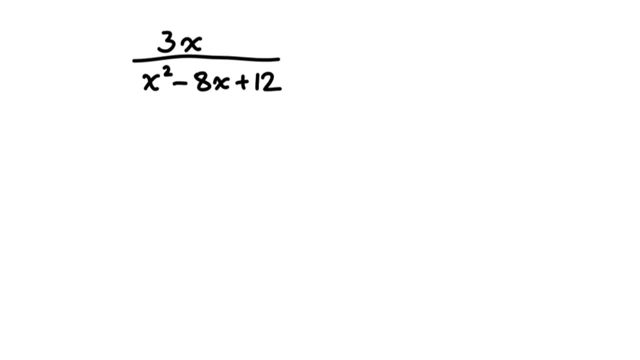 immediately state the restrictions, for you need to factor first. so in order for you to state restrictions on the denominator in the standard expanded form, you need to start with the standard expansion of the denominator and then start with the standard expanded form. so, for example, if you expanded form, you need to factor it. So this expression factors into. let's see the product.